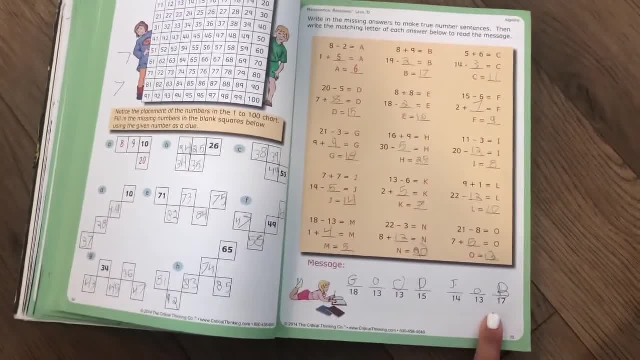 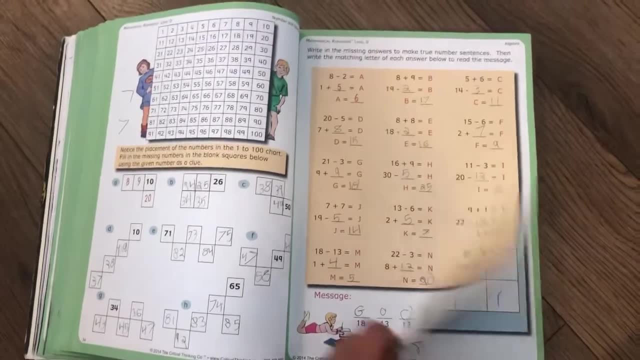 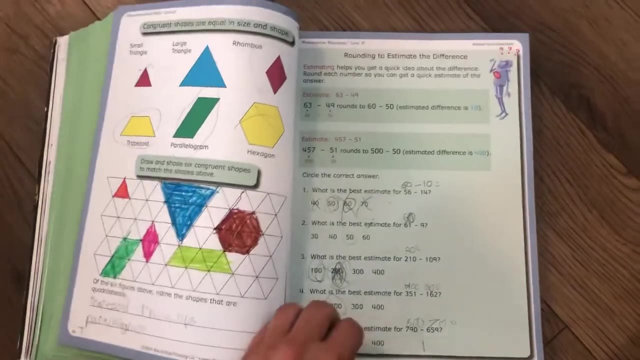 working, And so if you read the message and it doesn't make a word, you know you got one wrong, And so that's a really good tool for them to kind of self-correct and go back and know that they need to rework a problem. I've got some graphs and measurements rounding patterns. 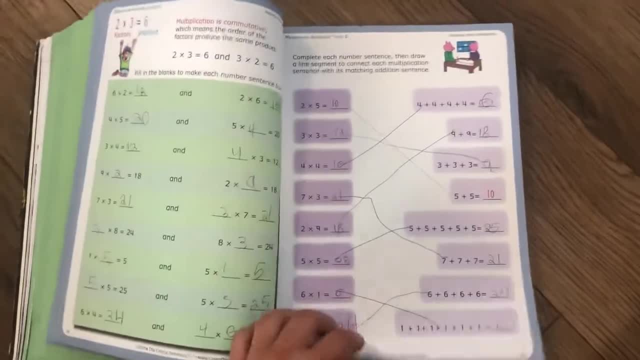 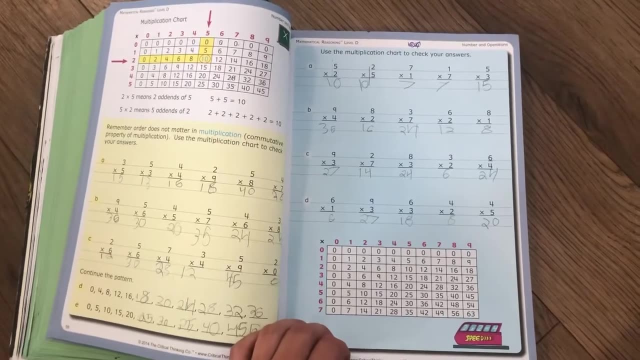 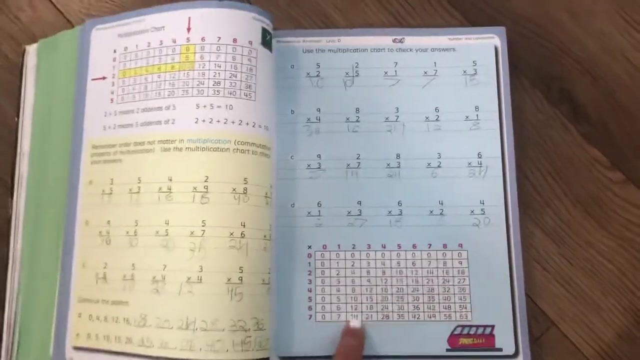 Time Multiplication is introduced. Lots of practice in here. We did do flashcards and drills separately as well. I really like my kids to master their multiplication and have it memorized, But these were great for introducing it. They felt comfortable doing it with these. 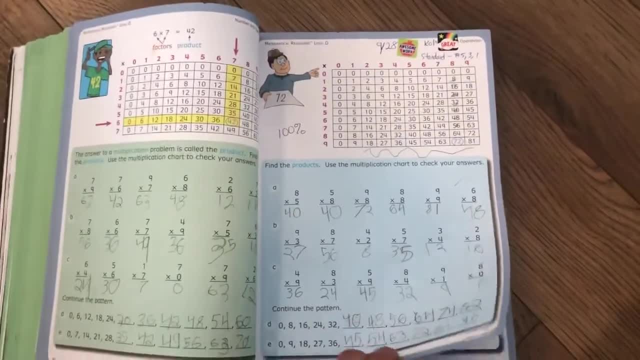 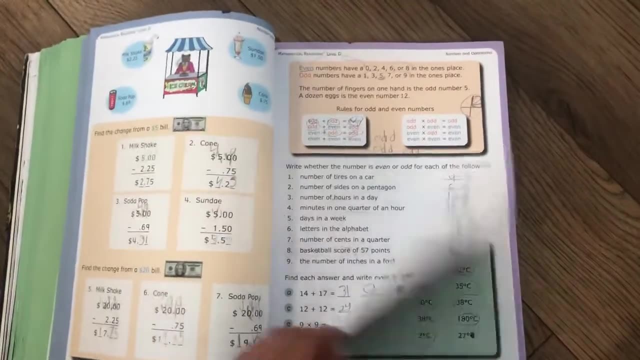 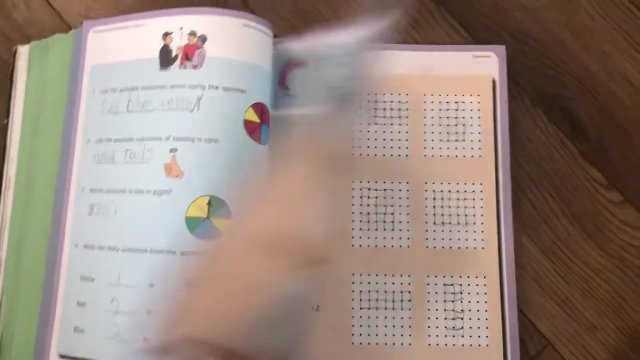 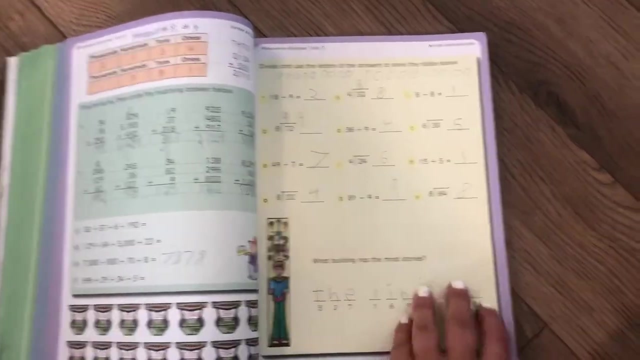 charts and getting that practice in. I like that. that was in the book More measurements and temperature Has metric And you can see. So one way to work this curriculum as well is you take how many pages are in this book and then divide it by the amount of weeks you're going. 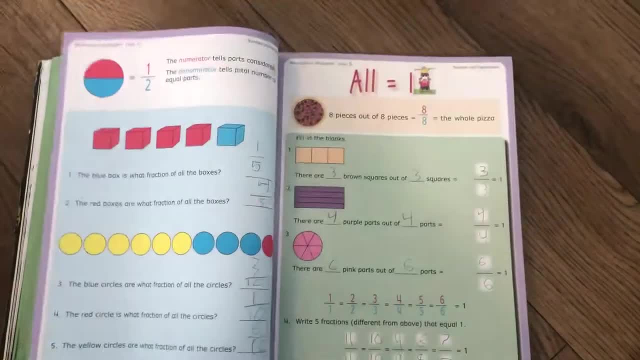 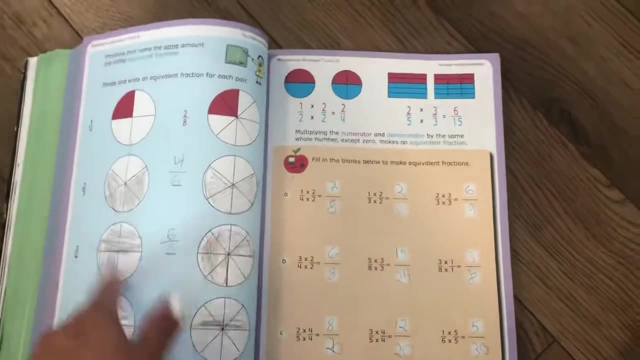 to do school, how many days you're going to do school a week, to know how many pages your goal is to accomplish. And I kind of would plan it out a week at a time and be like: okay, for example, like this is going to be easy peasy, We're going to find out how many pages we're going to do. 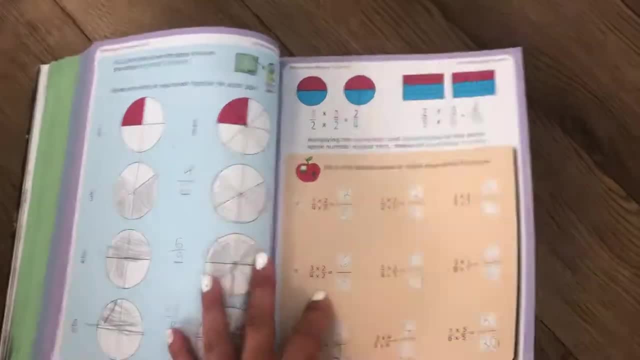 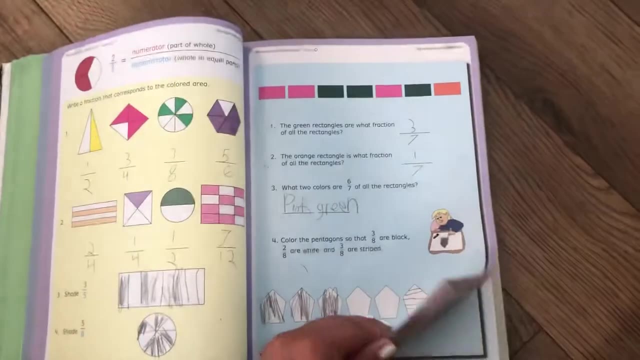 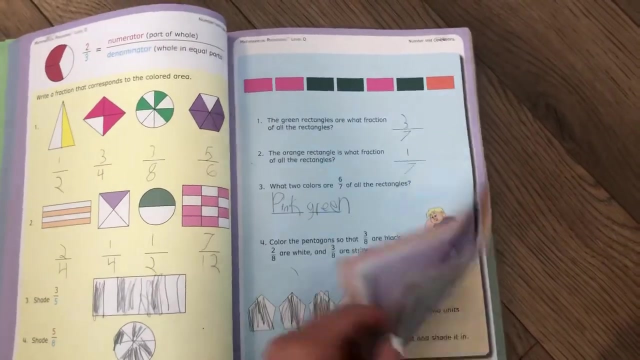 And then I will fly through that. So this we might do. we're going to do three pages this day, maybe four, And my boys sometimes I would never stop them, I at the bottom. Well, I must have done it in my other son's book, but anyways, I would write the letter of the day. 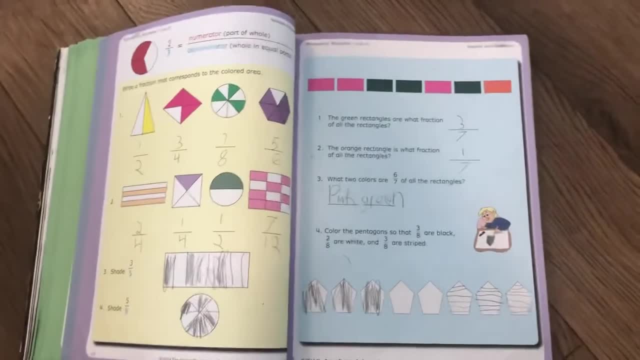 of the week- Monday, Tuesday, Wednesday- at the bottom of the corner. So we knew what the goal was. but if they wanted to keep working, we kept working. We allotted for about 30 minutes a day. They got to the. 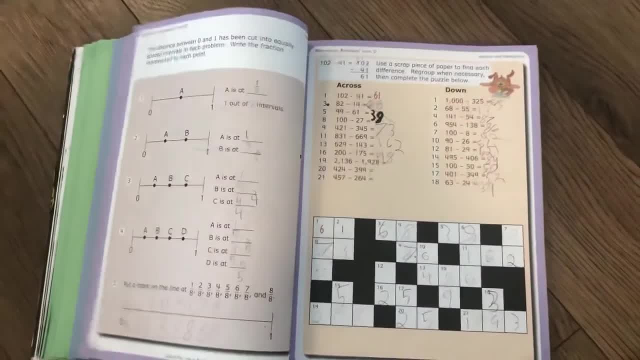 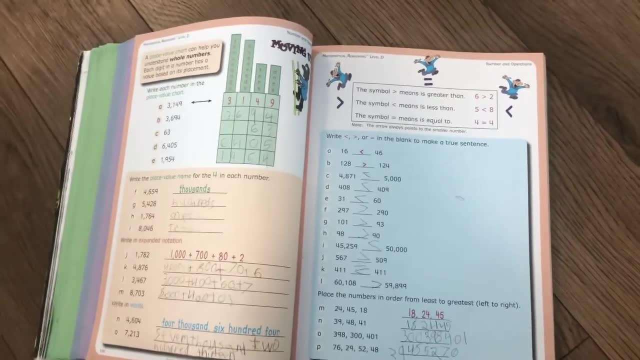 Two or three pages, Okay, And they were just done. We would stop if they were like, well, let's keep going. So I made it weekly goals so they knew if they worked harder. hey, we didn't have to do math on Thursday. 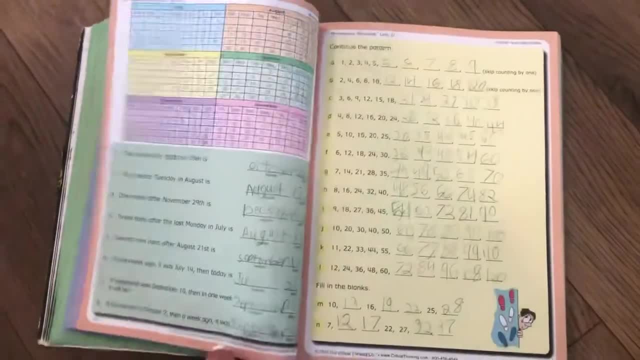 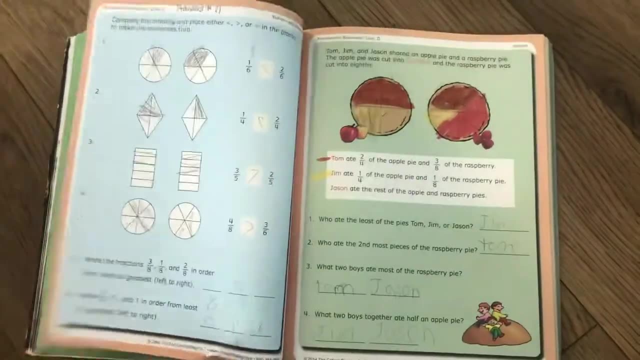 And we actually did finish a couple weeks even earlier than we were going to be done, because they just kept working. They enjoyed it a lot. Alrighty, as you can see some pages that I knew would be more difficult because there was a lot of problems. 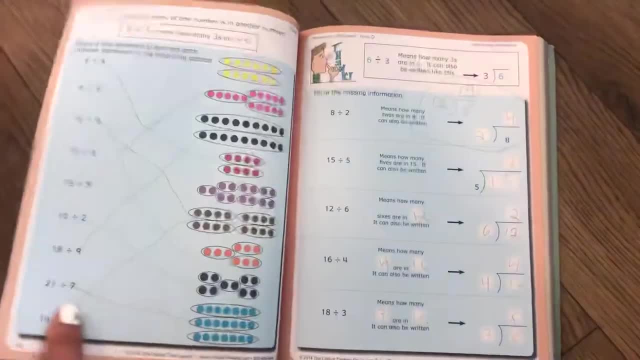 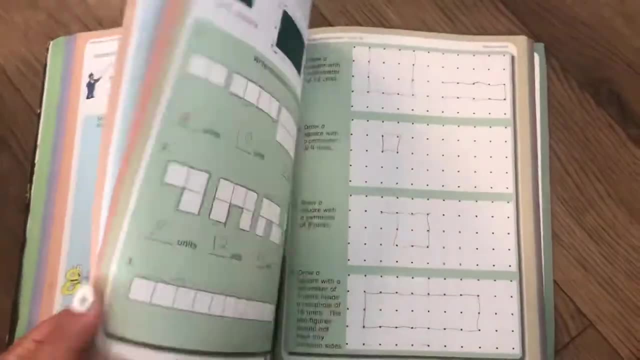 I maybe would skip a couple and add a fun page in there to give them a good variety. Like this is matching So they would do. that would be much easier than a page where there was a lot of adding and subtracting or something like that. that took longer. 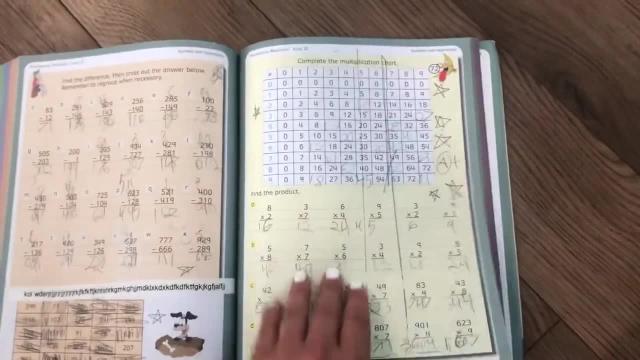 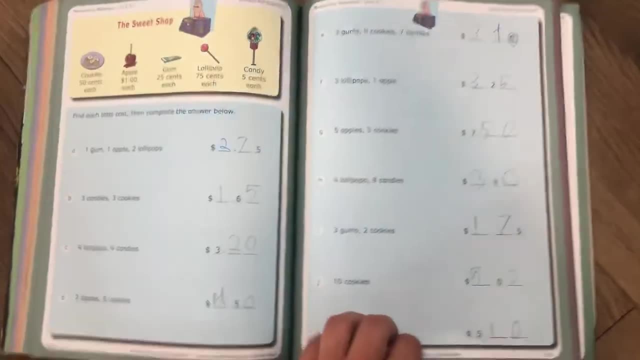 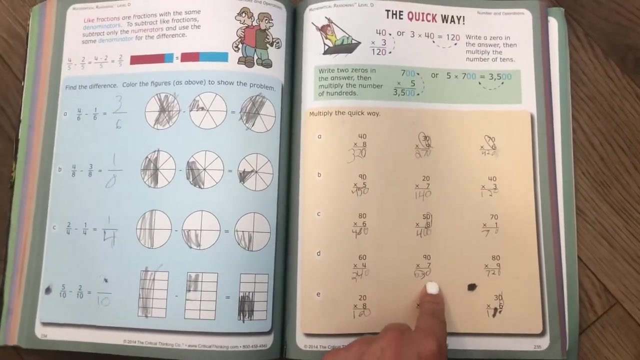 Like these pages, I would space this out. So if we did this, we would not do many more that day. Measurements, Money, Anything More difficult with the multiplication, And something I really require of my kids is to memorize their multiplication facts. 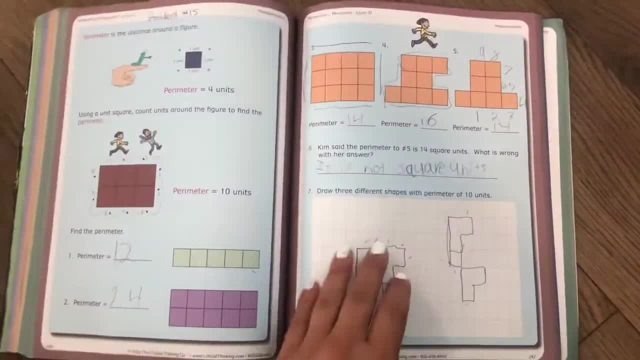 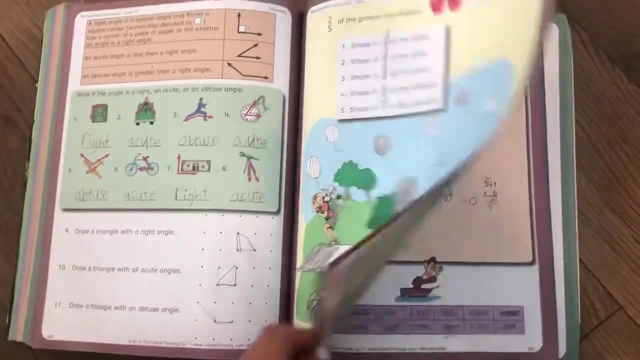 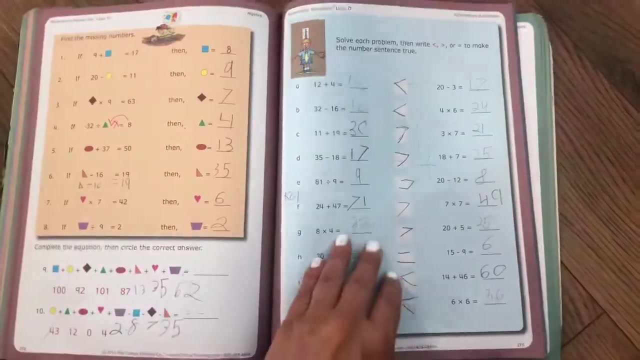 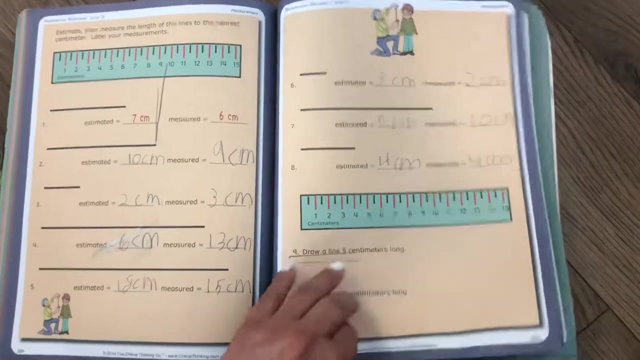 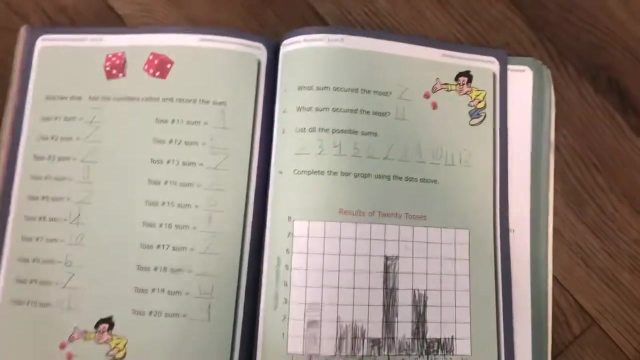 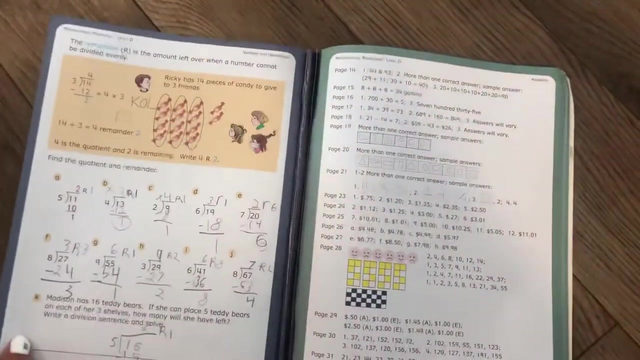 So we did, you know, much more drilling than this book had, which is our flashcards. We would spend a few minutes reviewing those throughout the weeks: Probability and graphs. They had a lot of fun. This was their favorite subject And at this level I don't feel like you really need much on a separate teacher's guide, because it's very basic. 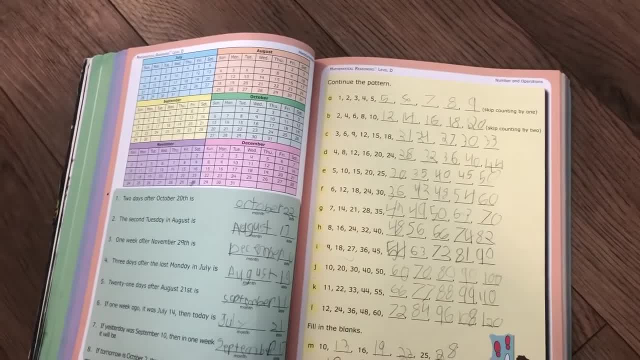 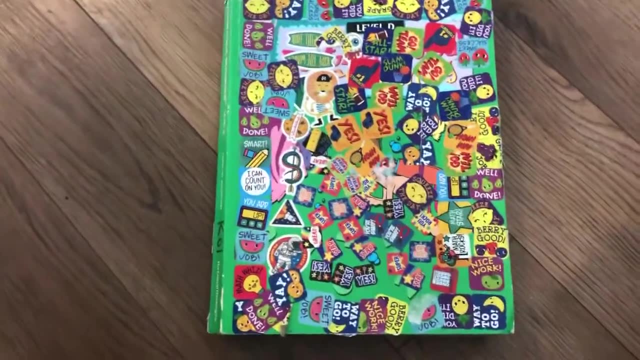 And so it just was an easy part of our school schedule last year to do math And it was positive And definitely adding the stickers on there made it a lot of fun. So I hope that flipped through It was helpful. If you have any questions, put them in the comments. All right, Have a blessed day. 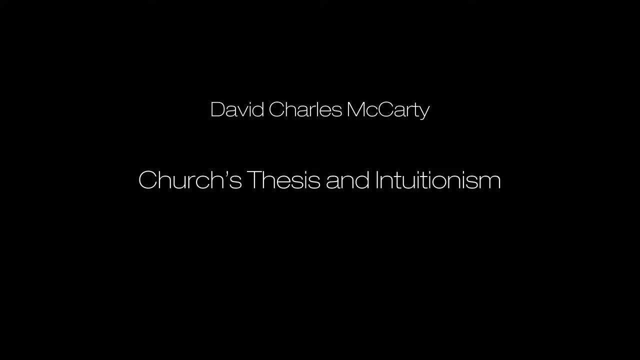 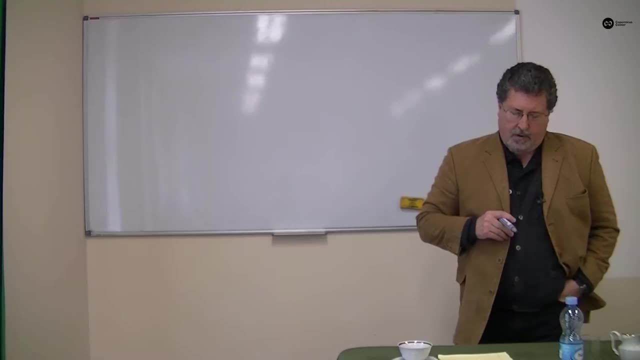 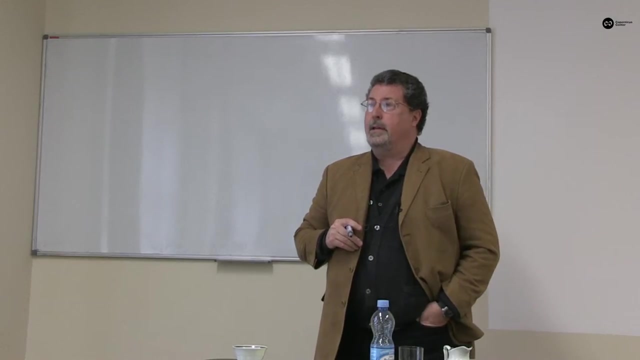 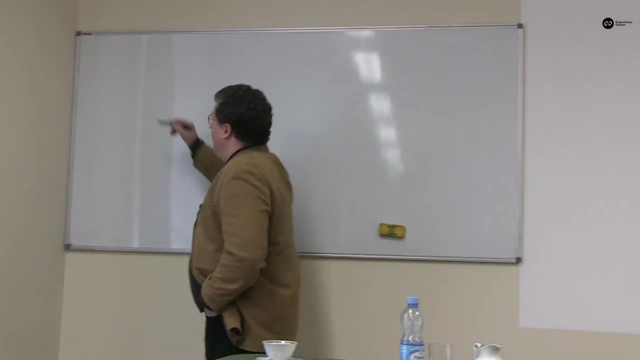 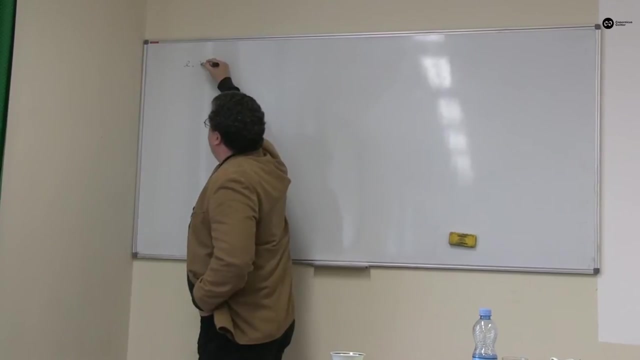 Apart from some standard intuitionistic assumptions, I am going to use one or two other assumptions only, or perhaps we might want to call them notational specifications. If I have a procedure represented by a natural number and I apply it to an input N, I'm simply going to write: